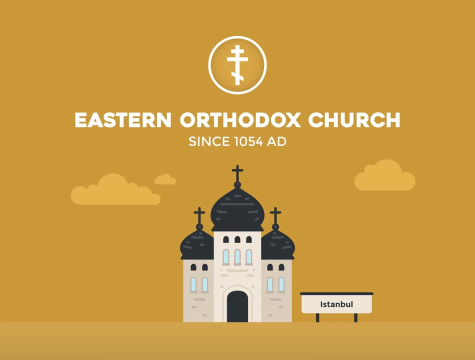 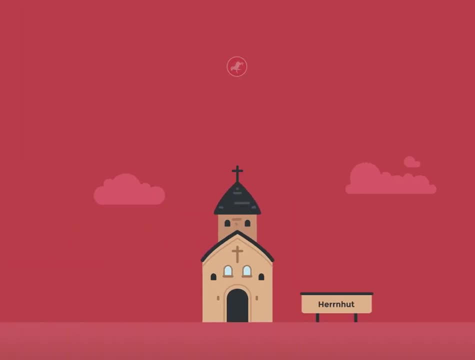 Eastern Orthodox Church, second largest Christian group with independent regional churches, focusing on traditions and rituals mainly found in Russia and Eastern Europe. Moravian Church emphasizes simplicity, missions and the spiritual unity of all Christians. Lutheran Church, first Protestant denomination, founded by Martin Luther, emphasizing faith and scripture over rituals. 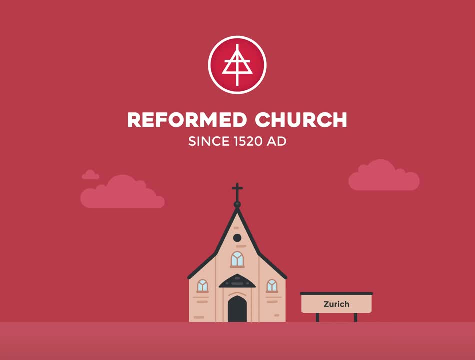 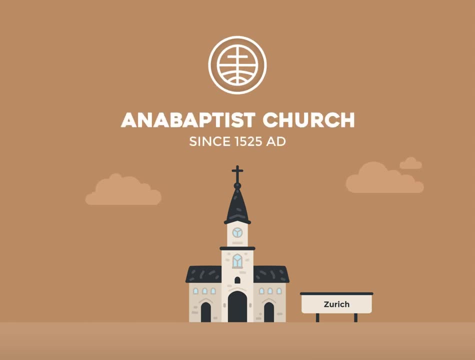 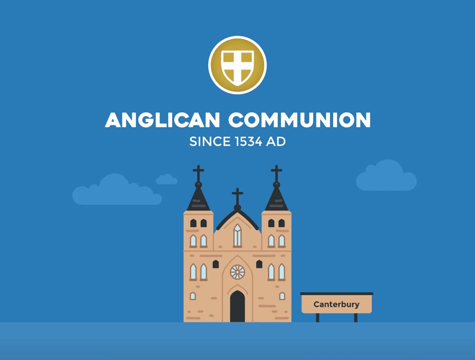 Reformed Church rooted in Calvinist theology emphasizing God's sovereignty and grace. Anabaptist Church: believes in adult baptism, pacifism and the separation of church and state. Anglican Communion- worldwide churches originating from the Church of England with a blend of Protestant and Catholic elements. 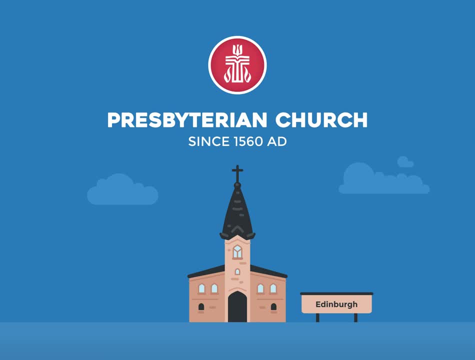 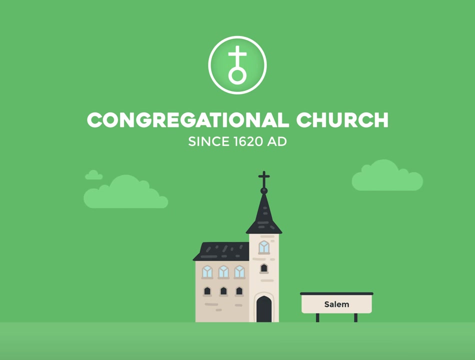 Presbyterian Church, governed by elected elders, emphasizes scripture and God's sovereignty. Baptist Church emphasizes adult baptism, congregational governance and the independence of local churches. Congregational Church, governed by local congregations, emphasizes autonomy and community involvement. Quaker Church values simplicity, peace and an individual's direct experience with God. 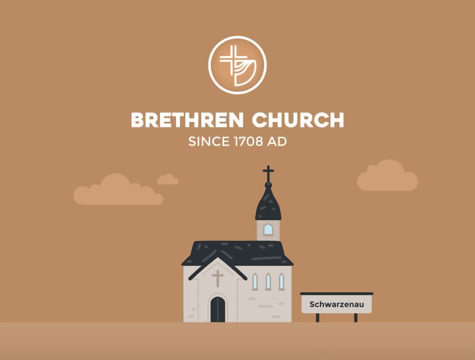 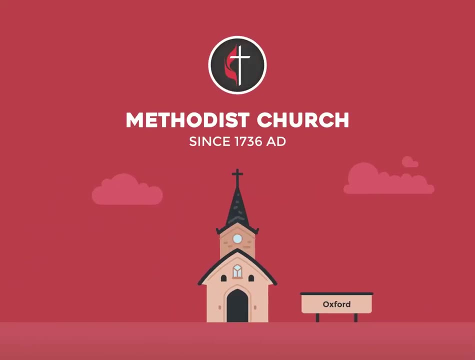 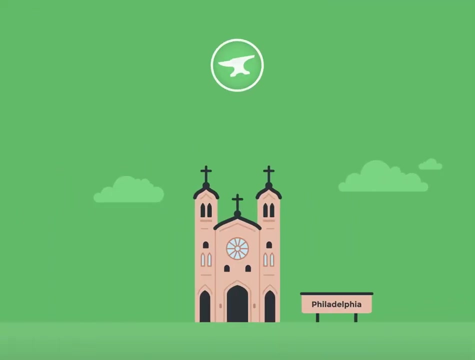 Brethren Church emphasizes simplicity, brotherly love and community decision-making. Methodist Church focuses on the importance of practical holiness, evangelism and social justice. African Methodist Episcopal Church, historically African American denomination with Methodist roots, emphasizes social justice. 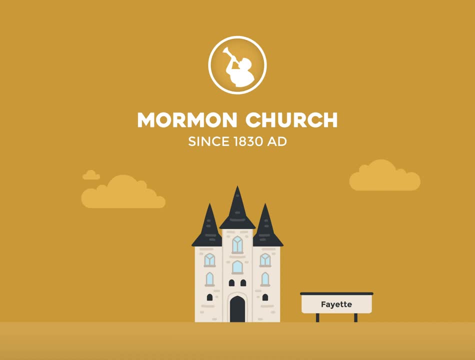 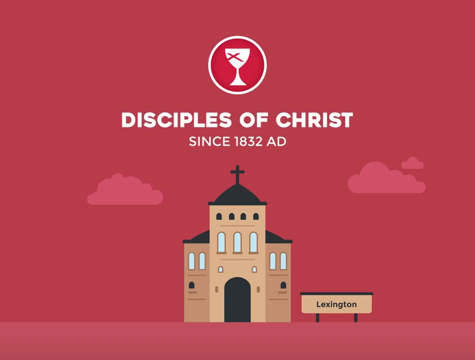 Mormon Church emphasizes the importance of the Church of God, Believes in additional scripture, the Book of Mormon and a continuing line of modern prophets, Disciples of Christ, values, unity, believer's baptism and the centrality of the Lord's Supper. 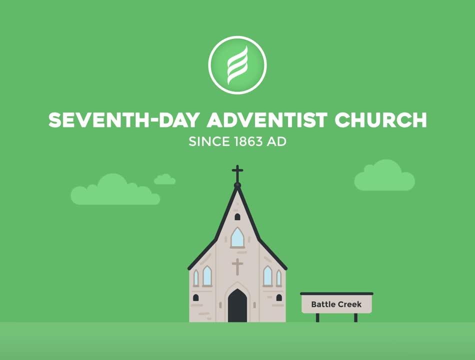 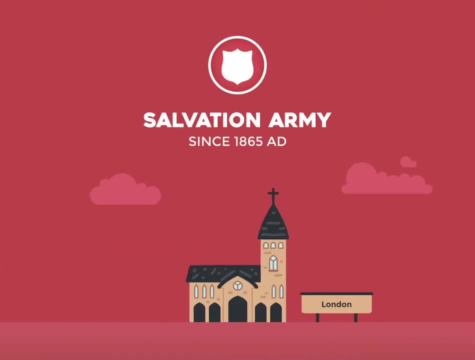 Seventh-day Adventist Church observes the Sabbath on a Saturday and believes in the imminent return of Jesus. Salvation Army Christian movement with a military structure focused on social welfare and evangelism. Jehovah's Witnesses predicts a coming earthly paradise. denies the Trinity and practices door-to-door evangelism.